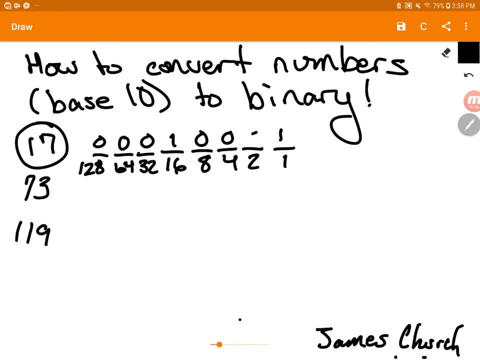 Everything else just becomes 0. And that's all there is to it. Let's do the sequence again with 73.. 1,, 2,, 3,, 4,, 5,, 6,, 7,, 8.. And then we're going to. 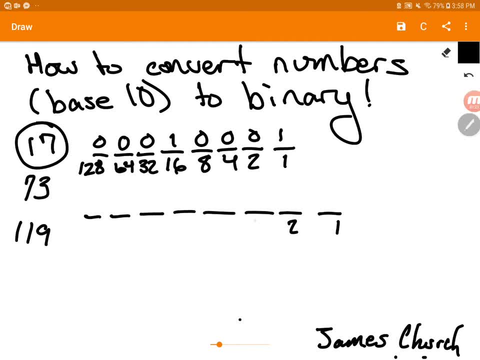 write our numbers: 1,, 2,, 3,, 4,, 5,, 6,, 7, 8.. 4, 8.. 16,, 32.. 64,, 128.. And then I come up with which numbers equals 73.. Well, I know, I'm going. 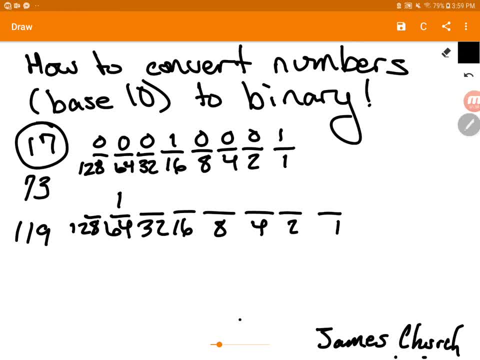 to need 64.. 73 minus 64 is 9.. I had to do that math in my head, So we know we're going to need the 8, and we're going to need the 1.. Everything else becomes a 0.. And now, finally, I want to do: 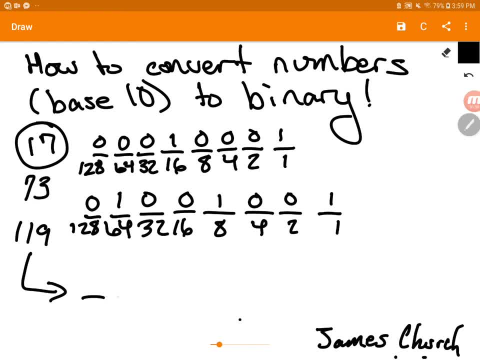 one more example. Let's do 119.. Let's do our 8 digits: 1, 2, 3,, 4,, 5,, 6,, 7,, 8.. And then let's write the numbers beneath them: 1, 2,, 4, 8,, 16,, 32,, 64,, 128.. All right, 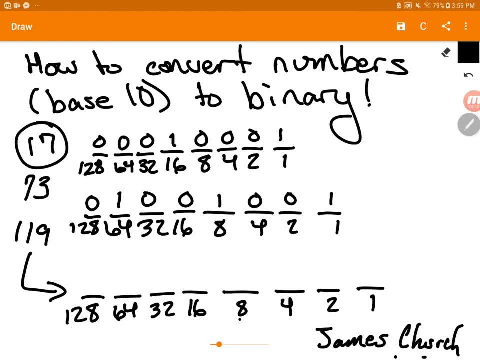 119 is less than 128. So I know I'm not going to need that one, But I will need 64.. And here's where you have to do a little bit of math in your head: 119 minus 64 is 55.. All right, So 55,. 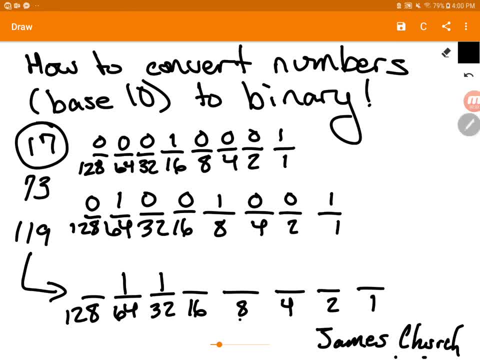 I know I'm going to need 32.. OK, So 52 minus- I'm sorry- 55 minus 32 is 23.. So I know I'm going to need 16.. And then 23 minus 16 is going to be 7.. And so, in order to get 7,, I do 4,, 2, and 1. And then everything else. 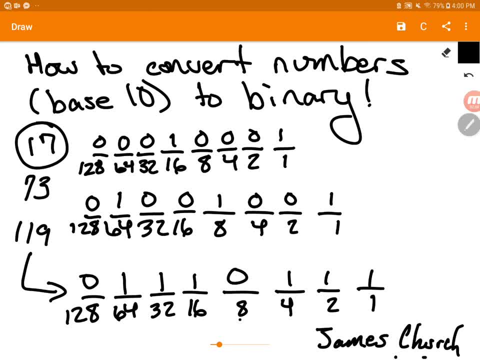 becomes a 0.. So we did three quick examples in this file. We did 17.. And there's the binary sequence. We did 73.. And there's the binary sequence. And there's 19. And there's the binary sequence. So here's the steps that we did. We drew 8 digits And then we did 1 to 128..